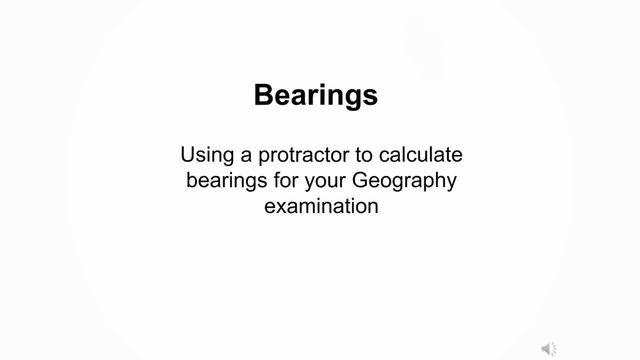 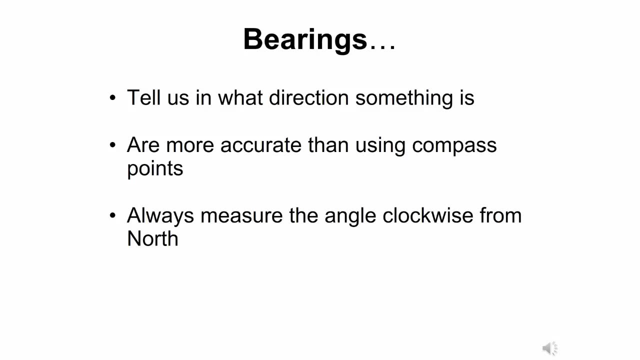 papers as well. When using bearings, there are a few things you need to know. first, A bearing actually tells us a direction. so when you're looking at a bearing on a map, you're looking at the direction that you're going. It's a lot more accurate than a compass point, whereas 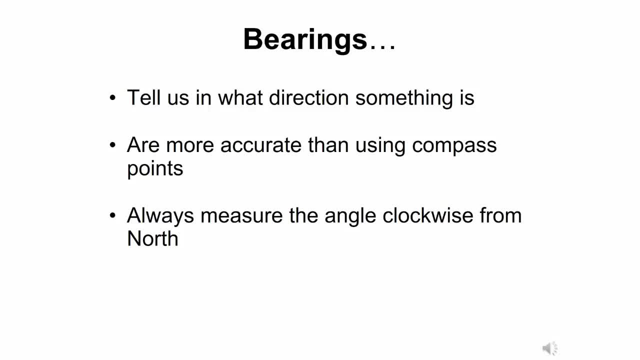 a compass point only tells you, for example, north-east- the direction that you're going. the bearing can tell you exactly the precise north-east direction that you're going to be going in. In addition to this, when you're measuring a bearing, you have to always start. 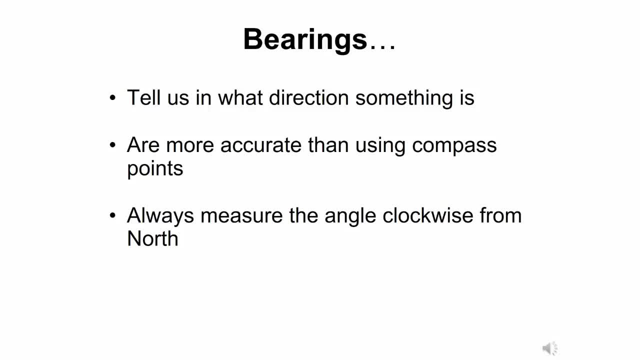 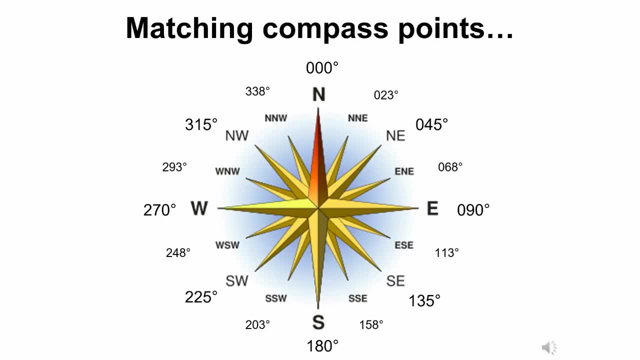 from the north and go around clockwise for you to get an accurate measurement. Over here you can see approximately what these bearings mean, especially compared to the matching compass points. For example, a north-east is approximately 45°, east 90°, south 180°, west 270°, and north is actually 0°. And if you were 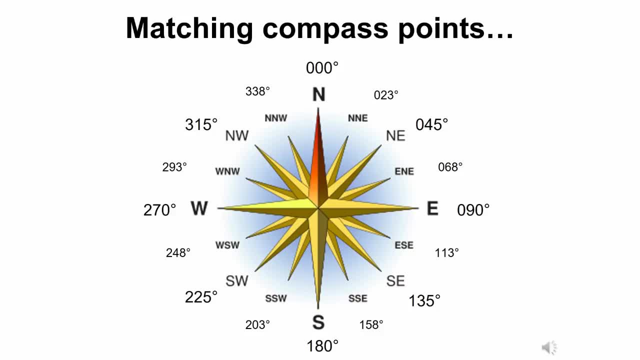 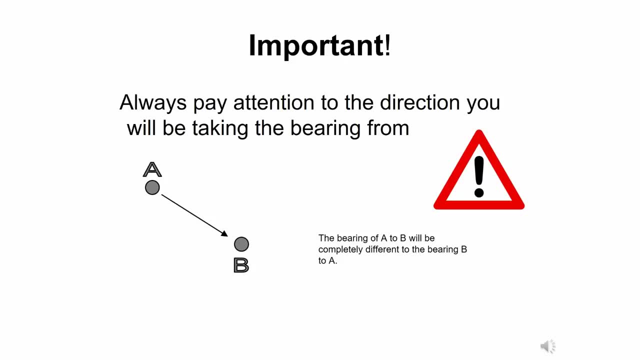 to fill in all the gaps. you can go down to a very, very precise direction. Now, for example, if you have two points, as you can see on the slide, point A and point B, and you ought to find the bearing from these two points, 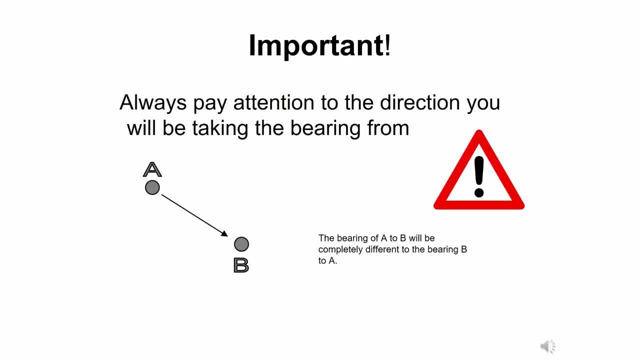 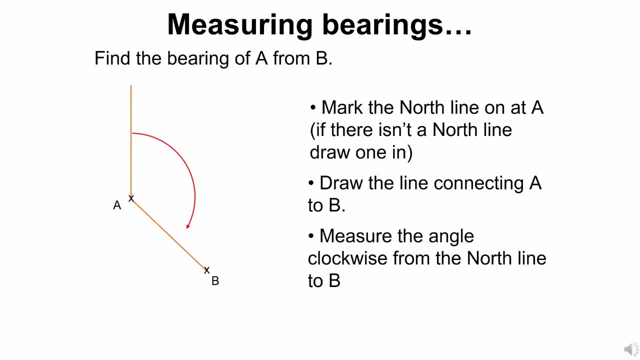 It's extremely important to read the question carefully and to figure out which is a starting point and which is a destination. for example, the bearing of a to b would be completely different from the bearing of b to a. so when it comes to measuring these bearings and you're wanting to find the exact degrees, 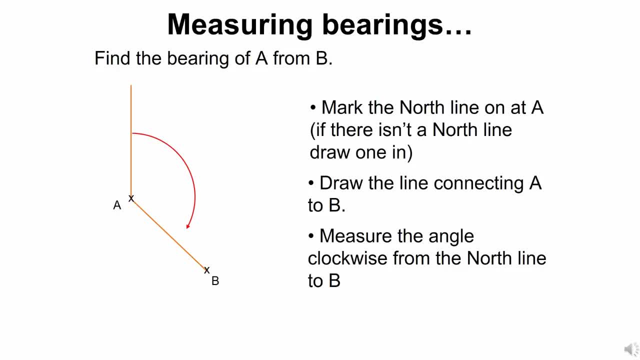 there is a certain procedure you need to follow. we are going on this diagram from point a to point b. the first thing you need to do is you need to draw a north line. the north line is a point leading from the point of origin a- in this case directly north um- to zero degrees. after we've drawn the 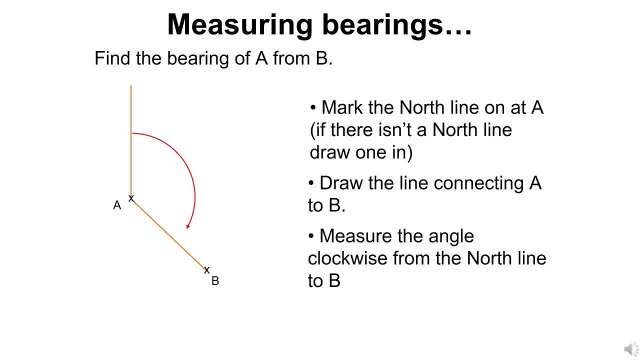 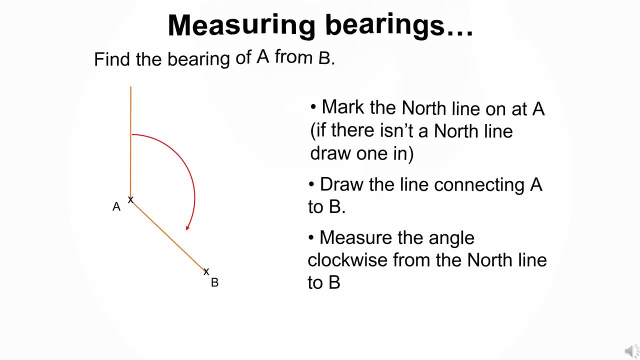 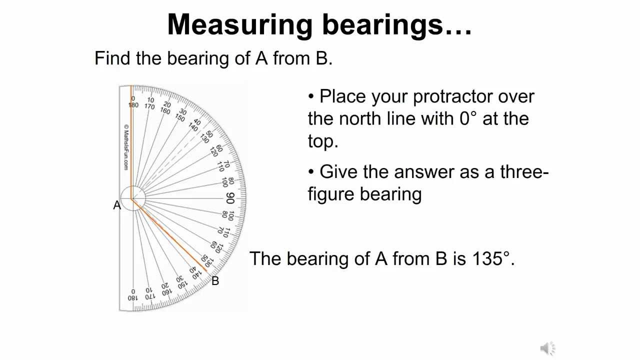 north line. you then need to connect the two points, the a and the b, and draw a line connecting them. you then measure the angle between the north line and the line that connects a to b, and this is your bearing. it is important to be very precise when calculating these bearings, so what you need to do is when. 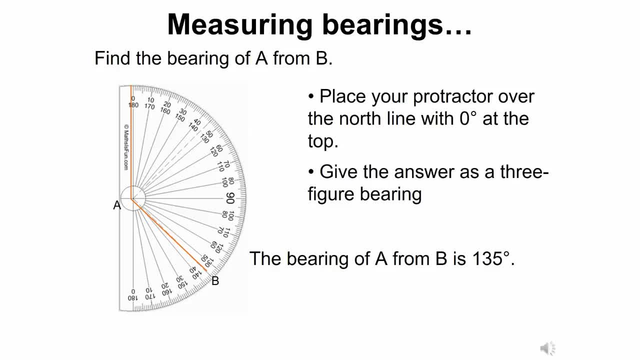 you've done all the points that i mentioned in the previous slide. you take your protractor. you make sure that the center of the protractor is exactly on the point where the north line intersects, the line connecting the a and b point. you make sure the zero, the beginning point of your protractor, 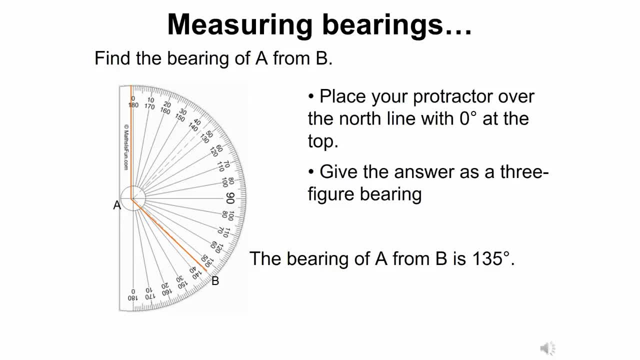 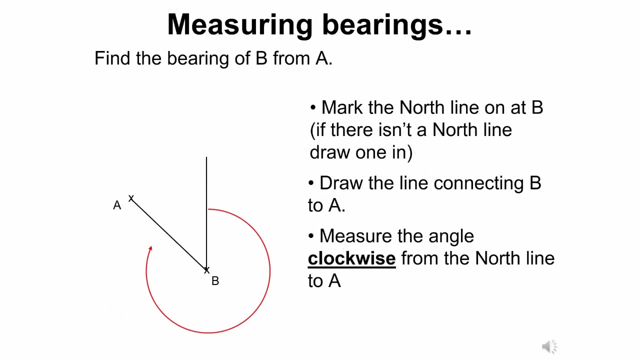 is on the north line and then you measure the angle around and you can see over here that the angle is just a little bit shy- of 135 degrees. that gives us a bearing of approximately, uh, south east, or more precisely 135 degrees. i mentioned previously that if you're looking at the bearing, it's very important to 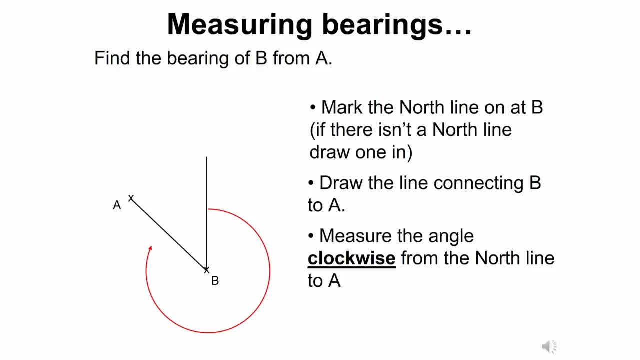 know the starting point, while these are exactly the same as the starting point of the protractor. so i'm going to draw the same line as the a and b, but this time, if i say i want you to find the bearing from b to a, notice we do it a little bit differently and the result is definitely not going. 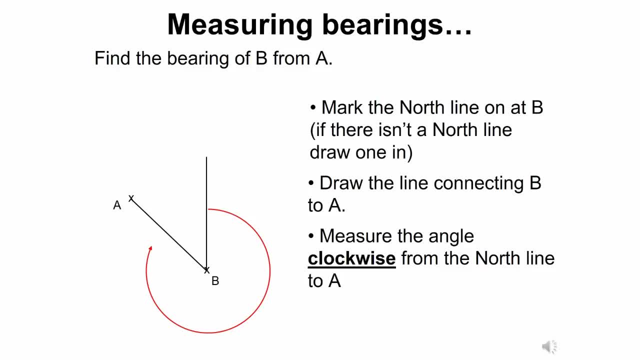 to be 135 degrees. so you follow the same procedure again: you draw a north line from the starting point, this case being b, and then you connect the b to the a and you want to measure clockwise going around the angle from the north line all the way to the line that connects the two points. 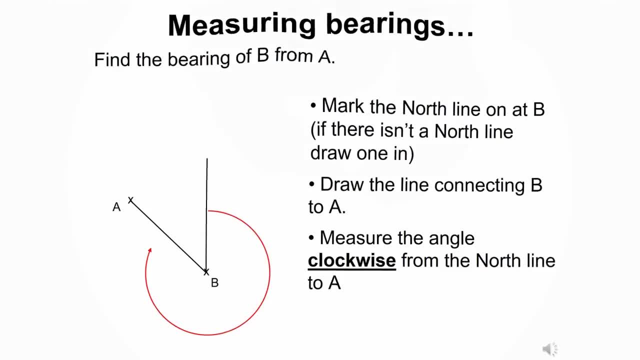 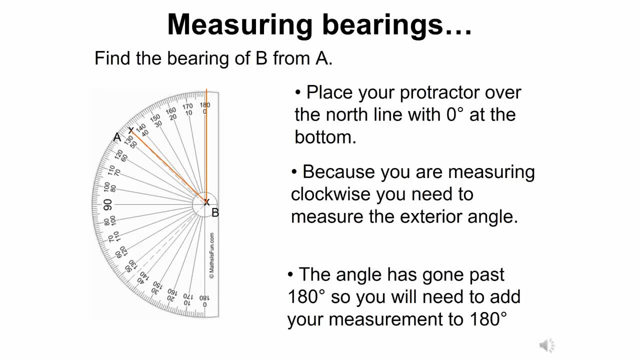 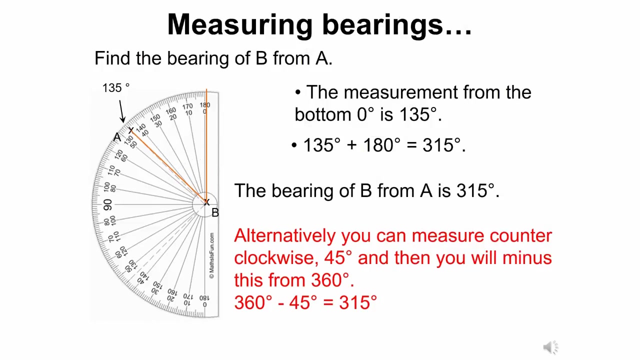 however, in this instance, you'll notice that when you place your protractor to measure these lines, you'll notice that the angle exceeds 180 degrees and therefore you have to do something a little bit different. in this instance, you're left with two different options. you can measure the angle again going clockwise, and you'll find out that the angle is 135 degrees.